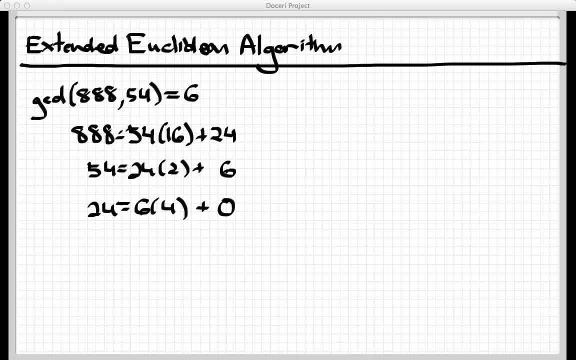 With a remainder of 24.. To continue the Euclidean algorithm, I shifted the 54 and the 24 into the previous spots for 888 and 54. So 54 is being divided into and 24 is now the divisor. We can quickly check that 24 goes into that twice with a remainder of 6. And I shift again and divide 6 into 24 and see that that goes in four times with a remainder of 0. Now the Euclidean algorithm says stop with the last number. 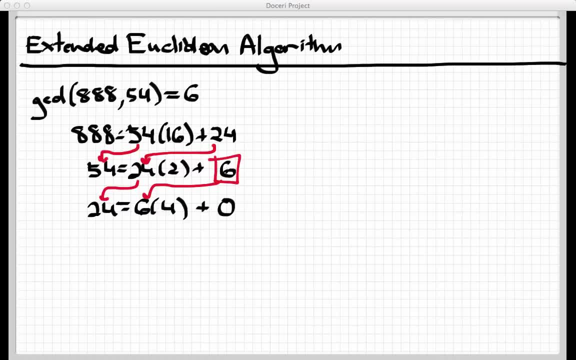 and the non-zero remainder. that will be right here and that's your GCD. So we're gonna use this fact that 6 is the GCD of 888 and 54, as well as the results of the process, to do something interesting with this GCD. 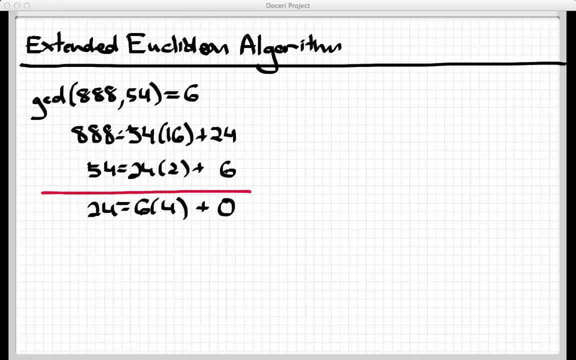 I'm gonna draw a little line right here and work with the two equations you see above that line, Starting with the number 6. here I claim that I can write 6 as a sort of combination of 888 and 54. Let me show you what I mean by that. 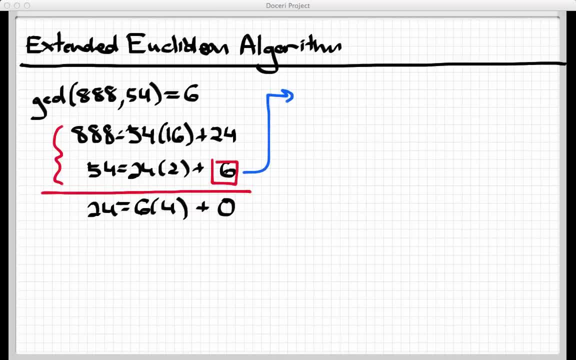 So I'm gonna start off by taking this equation and rewriting it in a slightly different form. I'm gonna write this as 6 equals. I'm gonna solve this equation for 6, basically. So 6 would equal 54 minus 24 times 2.. 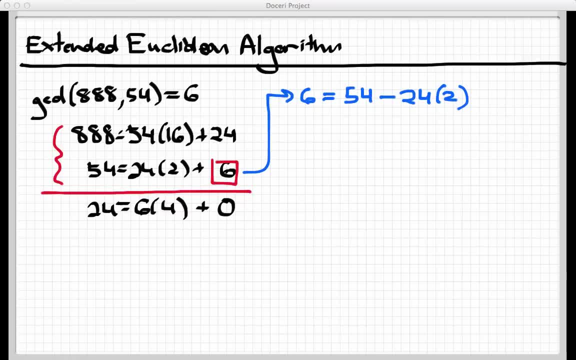 Now, certainly that's correct, because 24 times 2 is 48, and 54 minus 48 is 6.. I'm gonna rewrite this just slightly one more step here, and instead of saying minus 54 times 2, I'm gonna say plus 24 times negative 2.. 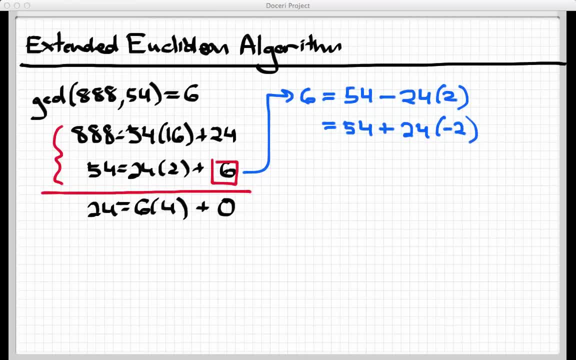 Now, interestingly, if I look up in the first line here, I see 24 hanging out in the remainder spot. Now I can solve that equation for 24, and 24 would be equal to 888 minus 54 times 16.. 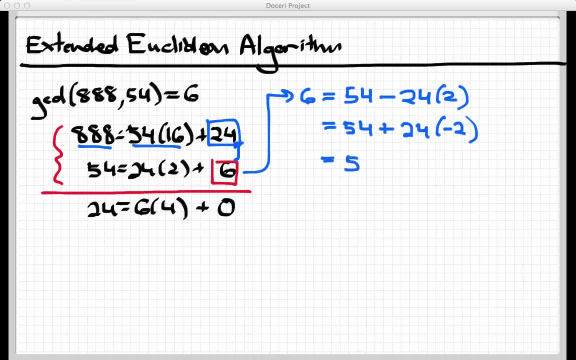 And I'm gonna put that into this equation over here where you see the number 24.. Let me put this in green: So 24.. I could also rewrite as 888 minus 54 times 16.. And that was being multiplied by minus 2 from the line up above it. 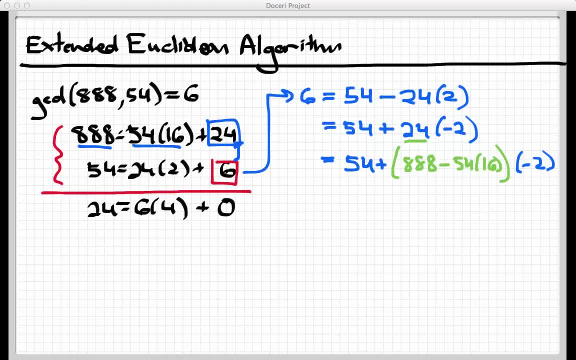 So basically, what I've done is I've substituted 24 with something that it's equal to. Now let me simplify some of the math here and explain what happens. Okay, so I have 54 in here, Inside the parentheses. I'm gonna do what I did a little earlier and say: this is 888.. 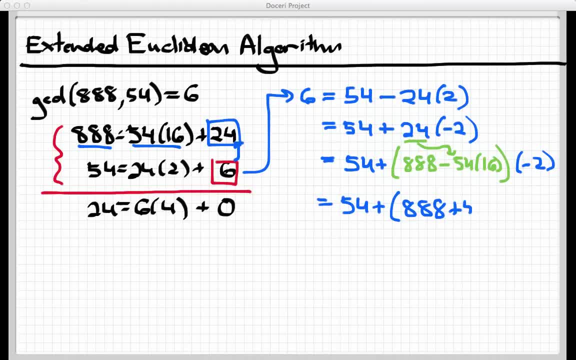 And not subtracting 54, but adding 54 times a negative 16. And the whole group there is multiplied by minus 2.. Now if I distributed that minus 2 through what I'd have here, I have a 54 here and I would have 888 times minus 2.. 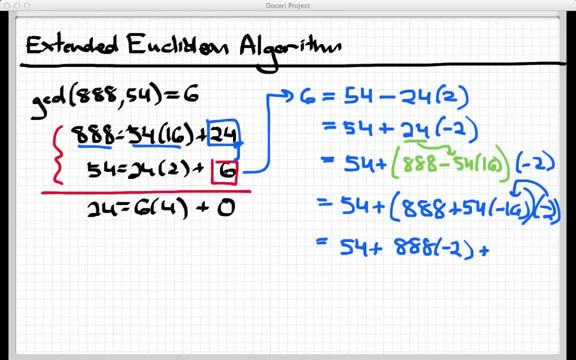 And then I'd have to multiply it to here as well. So that would be 54 times negative. 16 times negative. 2 is positive 32.. Now I have a 54 over here as well, So in the end I can write this as 54,. how many 54s do I have? 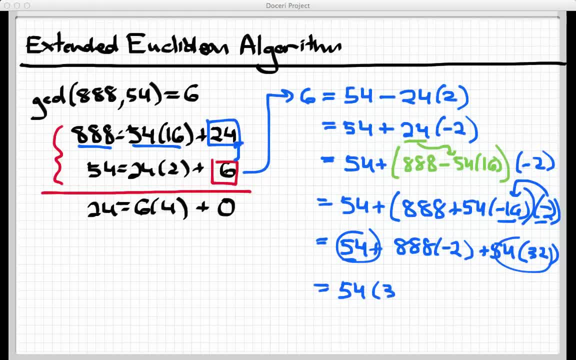 I have one here and 32 of them here, So that's 33 times or plus 888 times minus two, And this is all equal to six. Now you can check that this is true, but, importantly, notice what I've done here is. 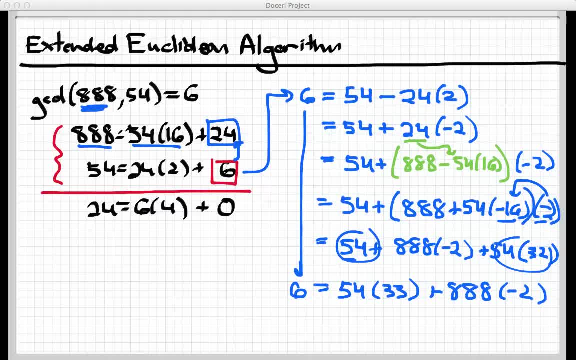 I started by looking this whole process. I started by looking at 888 times and 54 and found that their GCD was equal to six. Using the results of the Euclidean algorithm and sort of working backwards through the Euclidean algorithm by starting with that. 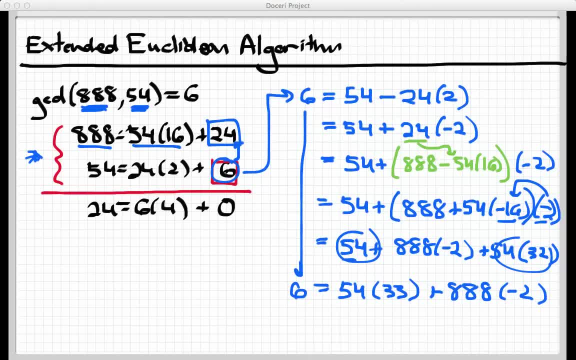 last non-zero remainder and successfully doing some solving and substitution, I've actually written six as a combination of 54 and 888.. I can take six and write it as 54 times an integer plus 888 times another integer. This sort of construction right here is called a linear. 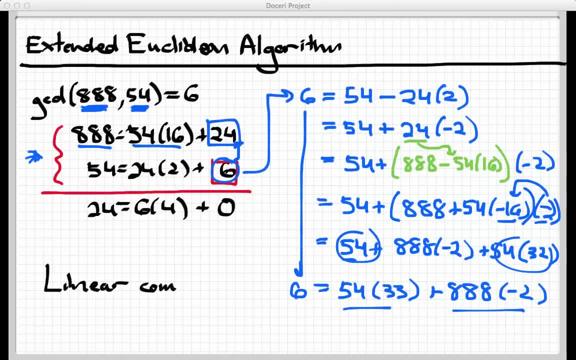 combination of those two numbers, 54 and 888.. What I've done here in forming a linear combination of these two numbers is I've taken 54 and 88 and multiplied them by integers and then added them. That's what a linear combination is. 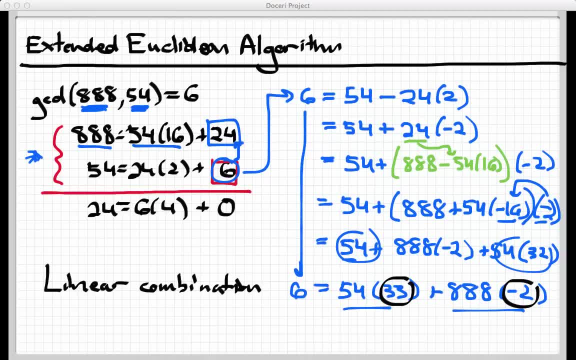 And what I see here is that the GCD of those two numbers is actually equal to a linear combination of the numbers that gave me the GCD in the first place. This turns out to be true for every pair of positive integers. you can find that the GCD of two integers 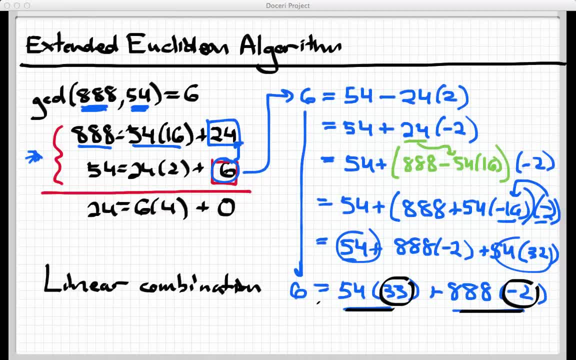 can always be written as a linear combination of those two integers. And the process that we just went through, this long process right here of finding the weights that I multiply these two guys right here, is called the extended Euclidean algorithm. So I can use the Euclidean algorithm to find the GCD in the first place. 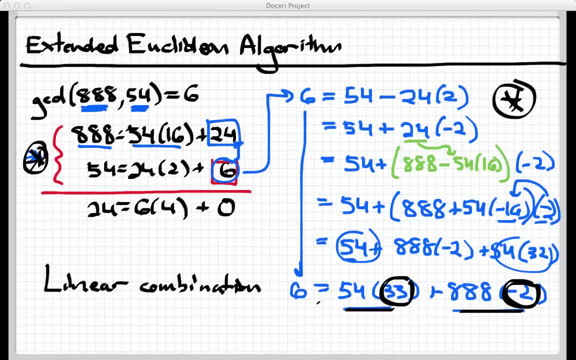 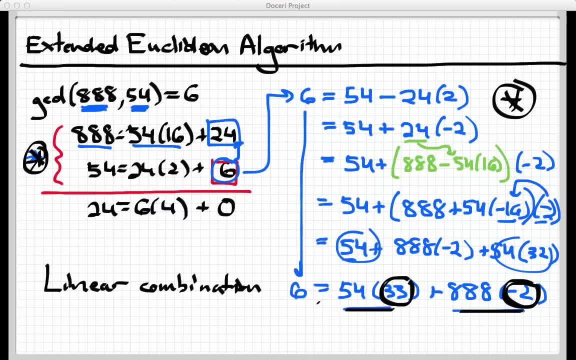 the extended Euclidean algorithm to write the GCD as a linear combination of the original two numbers. For for us that's going to be actually a very important process. So let's do one more example, actually as a sort of a two-stage example. 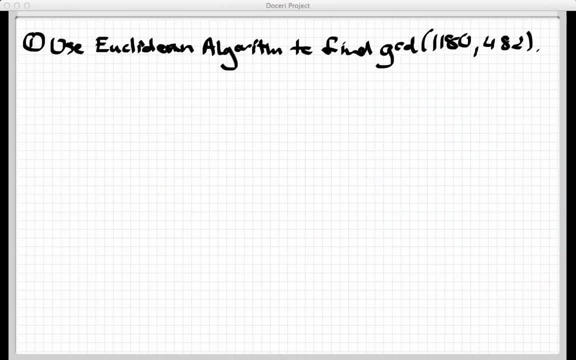 I'm going to look at the numbers 1180 and 482.. And first of all, I'm going to use the Euclidean algorithm to find their GCD When I do that. so this is another example of something we've already seen. 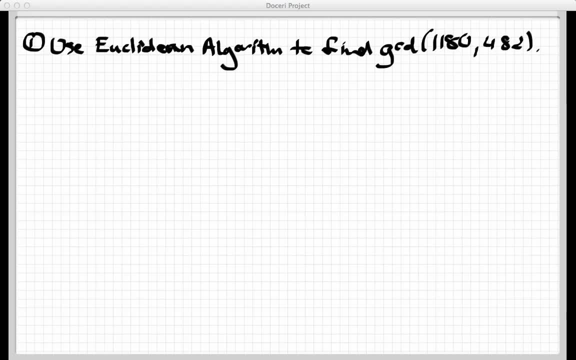 But, importantly, I need to keep track of the results here. So let's run through the Euclidean algorithm and see what happens. So the larger of the two numbers is 1180. So I'm gonna try to write 1180 as 482 times something, plus a remainder. 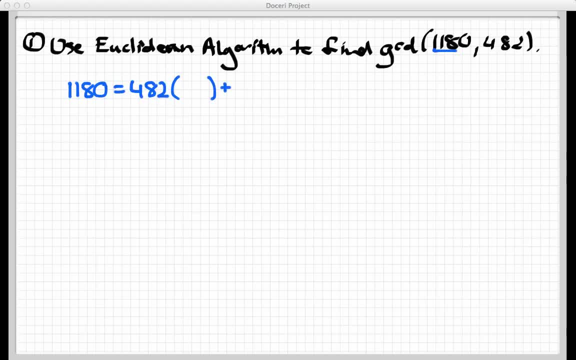 This is basically the long division, but I'm not gonna write the long division out. If you wrote it out as long division, you'd find that 482 goes in twice with a remainder of 216.. Now let's shift and see if I can find 482 equal to 216 times something. 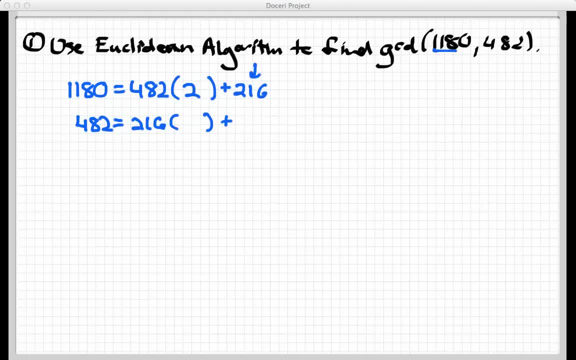 plus another remainder. This remainder right here was not zero, of course, and so the Euclidean algorithm hasn't terminated yet. Now 216 goes into 482 twice, with a remainder of 50, so I'm still not done. Let's shift them over. 216 is equal to 50 times something plus a remainder. 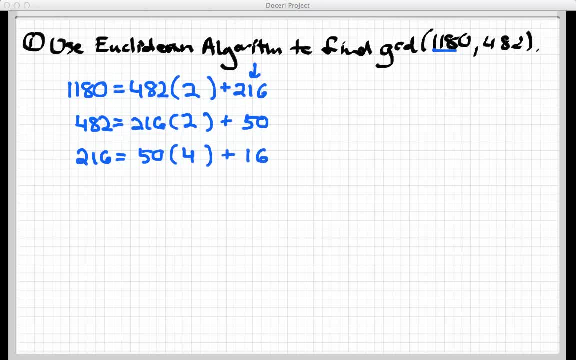 I can see that that goes in four times with a remainder of 16.. Still not a zero remainder, so I need to keep dividing. If I take 50 and divide it by 16, that is gonna go in three times with a remainder. 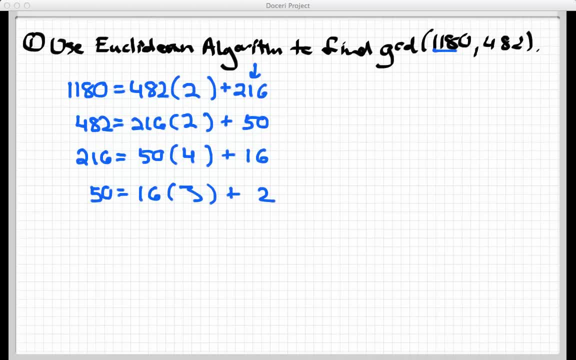 of two, that's still not zero. So I've got, I think, one more step to do with the Euclidean algorithm: Shift again and see if I can divide 16 by two, which of course I know how to do that. that's eight, with a remainder of zero. 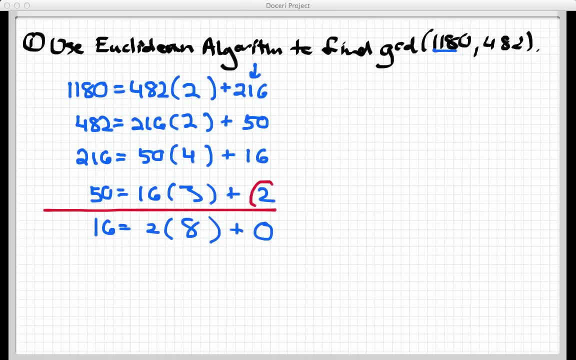 The Euclidean algorithm would say: stop here and look at that non-zero remainder, that last non-zero remainder. that's the GCD. So these two numbers have a GCD of two. So what we're gonna do now is use the extended Euclidean algorithm to write two. 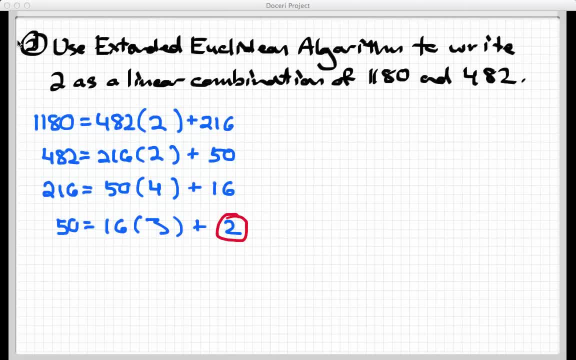 that GCD is circled in red there as a linear combination of 1180 and 482.. In other words, I'm gonna write, I'm gonna try to find two integers such that two is equal to 1180 times one of them. 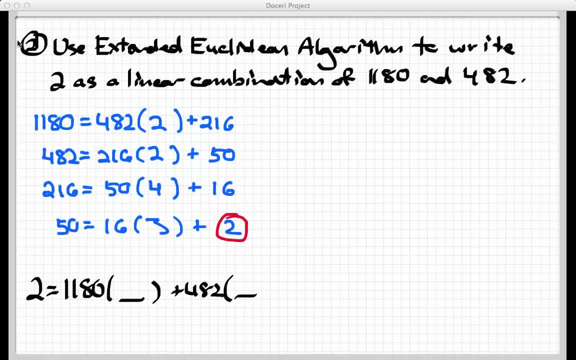 plus 482 times something else. Now, how we're gonna do that again is to start at the end of the Euclidean algorithm and work our way backwards. I'll do this in red, So let's first of all solve that last equation for two. 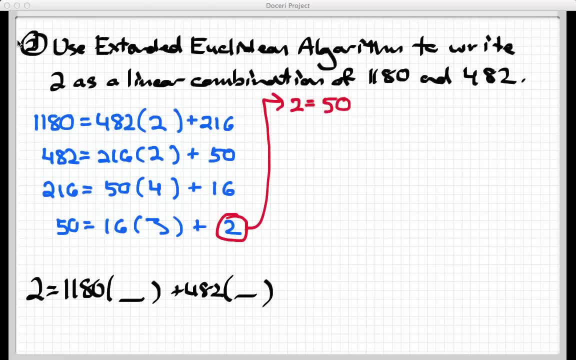 This is gonna be: two is equal to 50 minus 16 times three. But I'm gonna write that as plus 16 times negative three. Again, I've just taken that last equation on the bottom there in blue and solved it for the number two, the smaller number there. 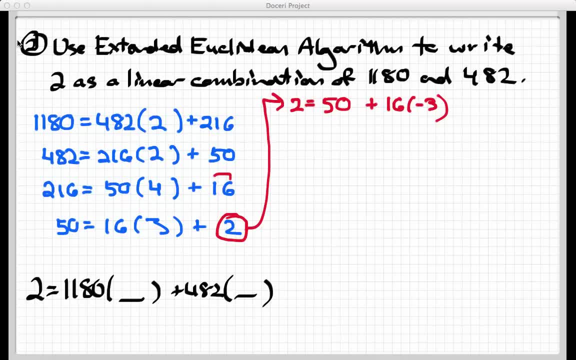 Now, if I work my way up the chain here, what I see is that 16 can be written as 216 minus 50 times four. So I'm gonna substitute this 16 right here with something that it's equal to. So this is 50 plus. I'm gonna make a substitution that's gonna equal 16.. 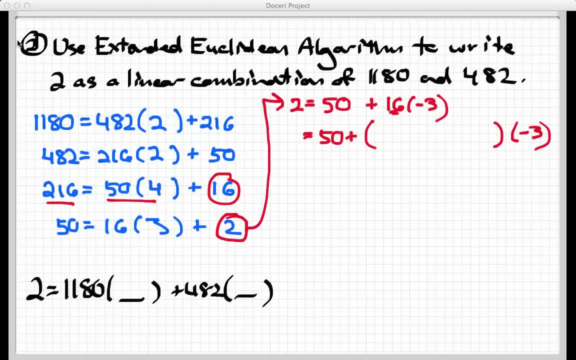 I'm already multiplying the 16 times a negative three, So what goes in here? that is gonna be 216 plus 50 times negative four. Now let me distribute the three through and notice what's gonna happen here. I'm gonna have 216 times negative three and 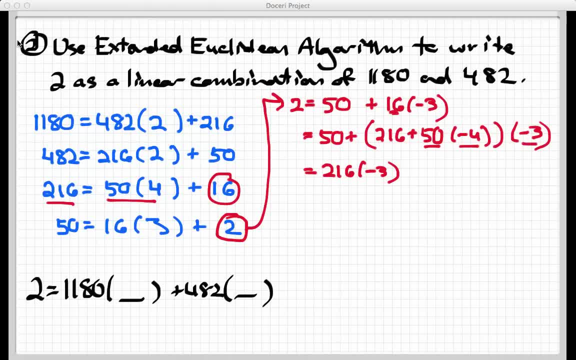 then I'm gonna have 50 times negative, four times negative three. That's 50 times 12, and then I have another 50 hanging out over here. So in all that becomes 50 plus or 50 times 13.. 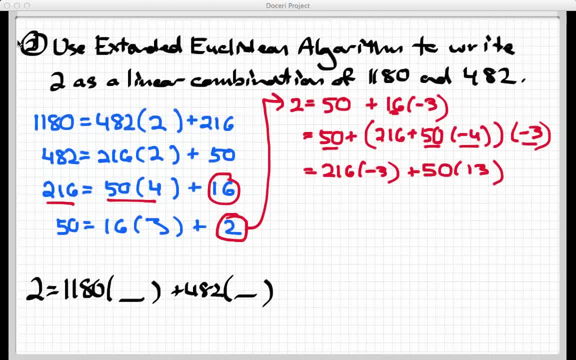 And if you stop right here and just computed this right-hand side, you would see that it equals two, and that's a useful check. Okay, so now I notice that 50 right here can be written as 482 minus 216 times two. 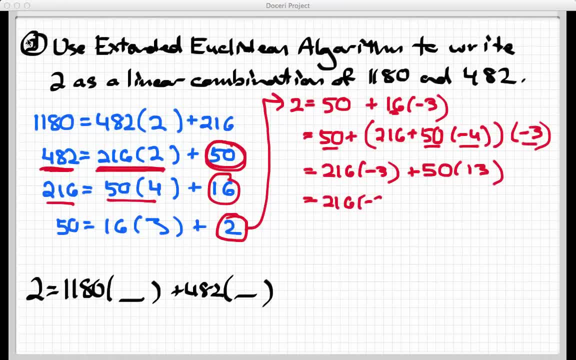 And so I'm gonna do a substitution here of the number 50 that you see right there. So I'm gonna create a space for the substitution, keeping in mind that I'm already multiplying all that stuff by 13.. Now, according to the second line of my Euclidean algorithm, 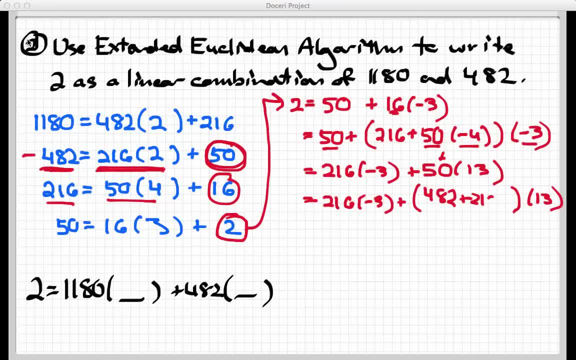 50 is equal to 482 plus 216 times negative two. Now let's check things out here. I have 216 times negative three, and then I also have 216 times negative two times 13. So how many 216s is that in all? 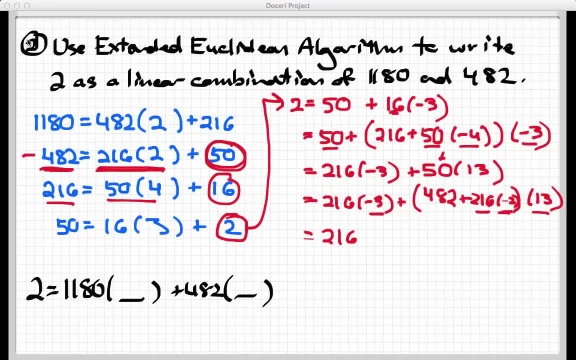 Well, I had negative three right here and I'm gonna have negative 26 right here, So this is a total of negative 29 times 216.. And the 482 is also gonna be multiplied by 13, once I distribute this 13 through there. 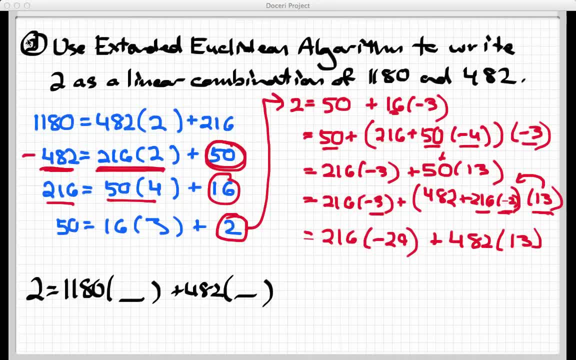 So you can stop right here and check that this side right here does actually equal two. Now one last substitution step. okay, The 216 here can be written as 1180 minus 482 times two. So I'm gonna do one last substitution and then I think we'll be close to done. 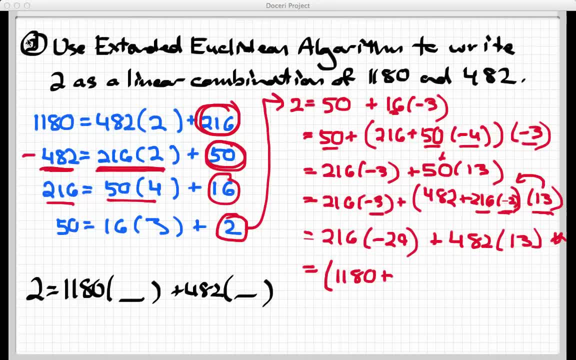 The 216 is equal to 1180 plus 482 times a negative two, All times negative 29.. And this is also all plus 482 times 13.. So now let's see where we end up here If I distribute this negative 29 through. 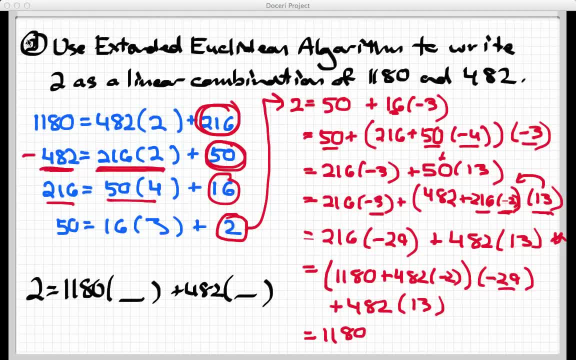 what I end up with here is I have 1180 times negative 29. And a lot of 482s negative. 29 times negative two is 58.. And I have that many 482s here. 58 plus 13 is 71..